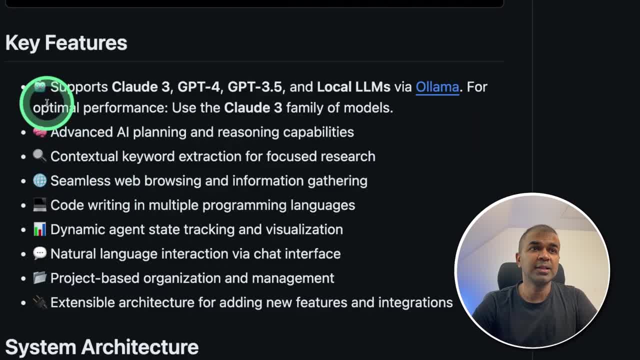 open source large language model using Ollama. You can see it supports Cloud 3,, GPT-4,, GPT-3.5 and local models via Ollama. advanced AI planning and reasoning capability, contextual keyword extraction, seamless web browsing, code writing and a lot more. Let's get started. 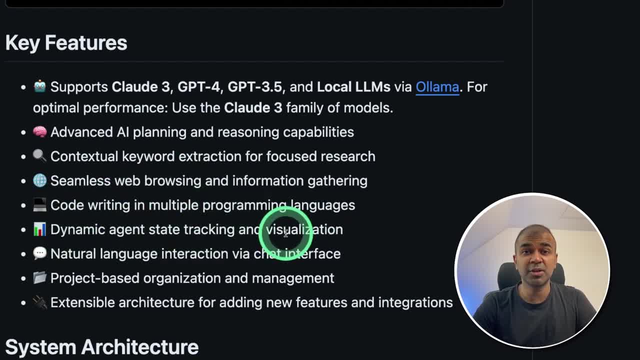 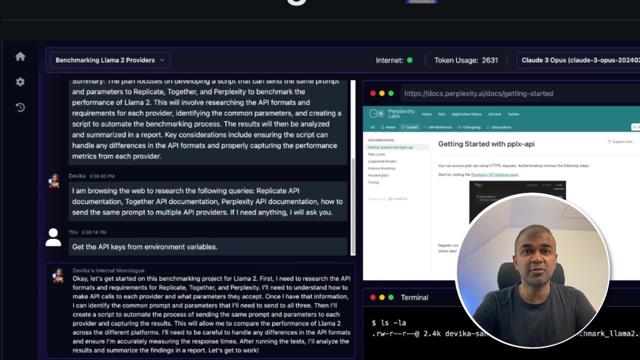 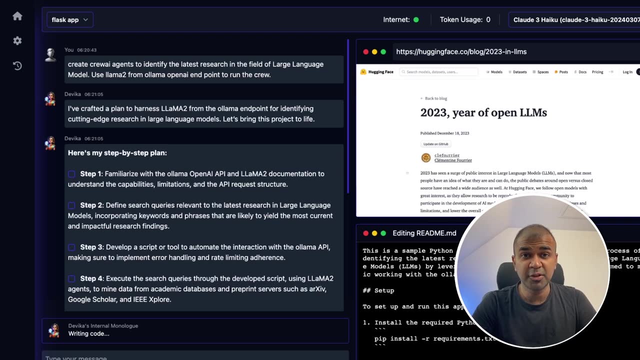 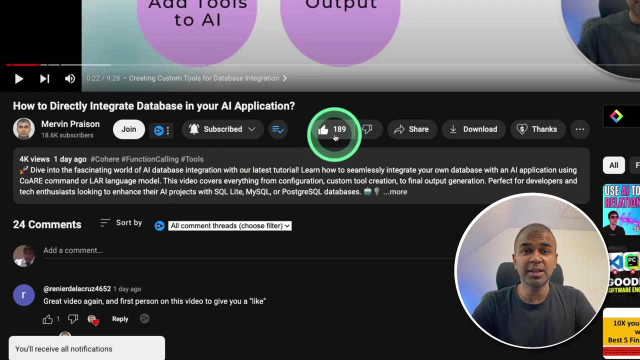 I'm going to take you through step by step on how to install this on your computer and test this, But before that, I regularly create videos in regards to artificial intelligence on my YouTube channel, So do subscribe and click the bell icon to stay tuned. Make sure you click the. 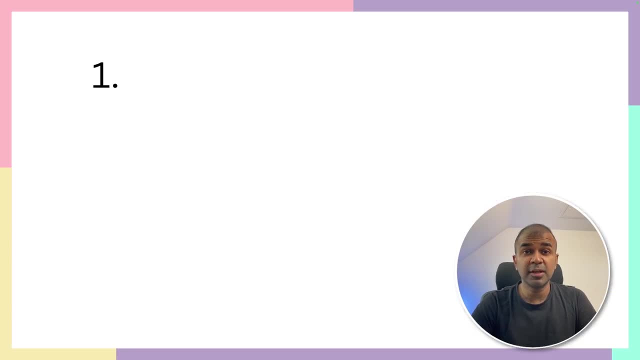 like button, so this video can be helpful for many others like you. In this we are going to see how to configure this and how to configure it. Let's get started, Let's get started, Let's get started. Then how to set up the front end, then how to set up the back end. In this we are going to run two. 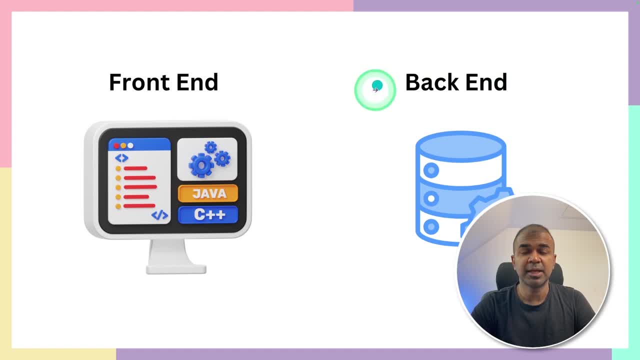 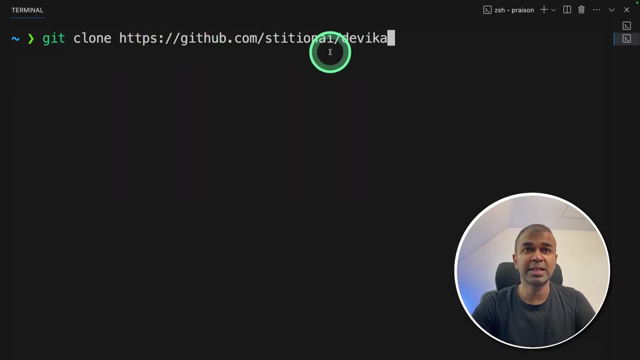 softwares. One is Flask, written in Python. That is the back end, So we will keep that running And in the front end we will use Bun. It's a JavaScript based front end application, So that's what we see in our browser. So first step, git clone and the GitHub URL, slash Devika and then click enter. 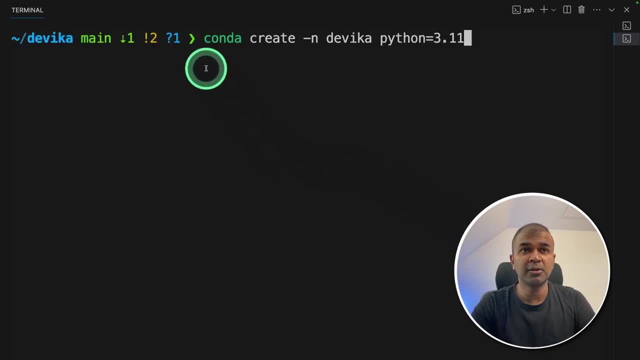 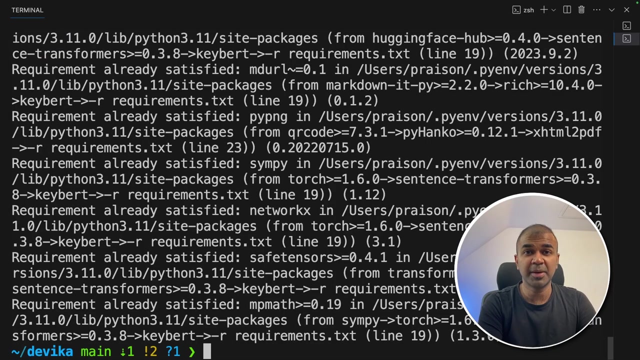 Next navigate to the Devika folder. Now conda create hyphen- and Devika- Python equals 3.11- and click enter. Now conda activate Devika and then click enter. Next pip install hyphen- our requirementstxt, and then click enter. This will install all the required dependencies or the 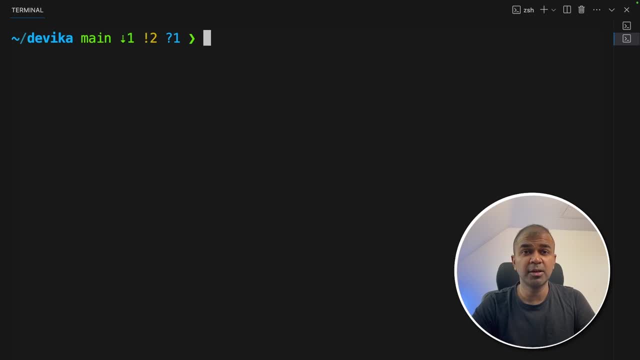 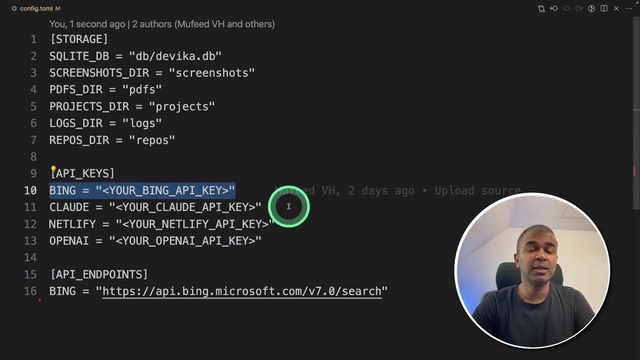 packages. Now, if you open this code folder in VS Code, you can see various files Among that. we need to change configtoml. Just open it. It will look like this: So here you got API keys, So you can use cloud API key. If you're using OpenAI, you can use OpenAI API key, So replace this. 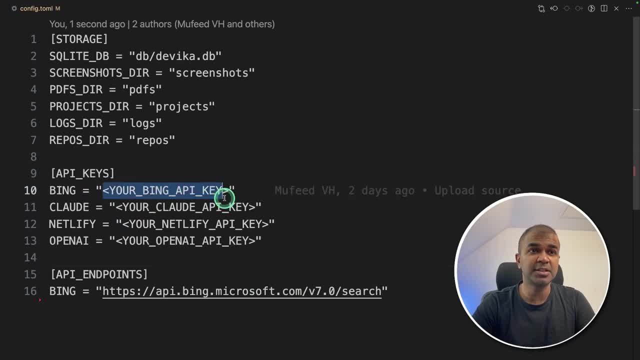 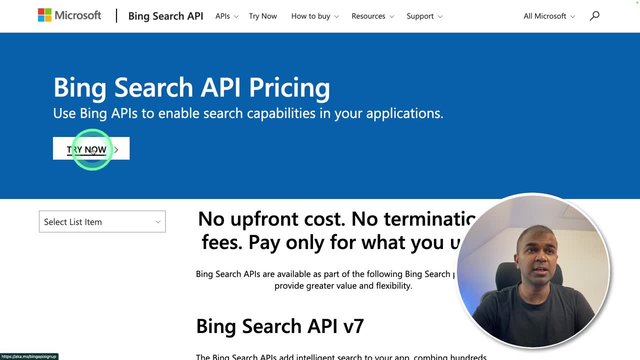 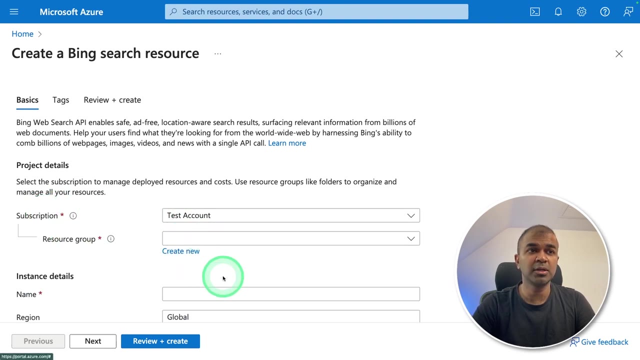 accordingly. One difference is that for Bing search API key you might need to follow different steps. So you got the Bing search API page There. you can click try now. There you will be presented with a page like this: Enter the subscription resource group or you can create a new one. 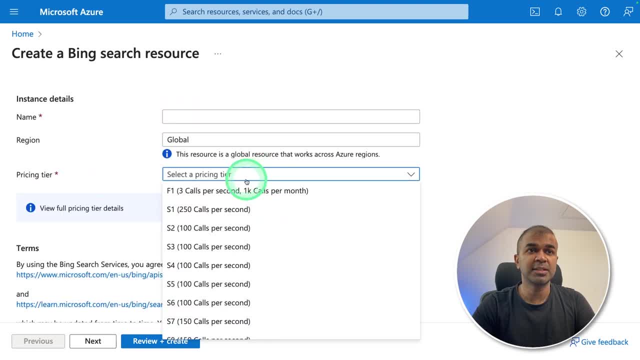 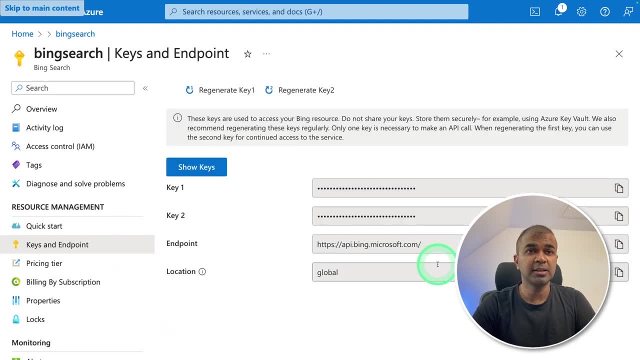 Then provide a name for the instant Select the pricing tier So you can choose the first one for basic tests, Then confirm and you can create it Once. after you create, you will have a page like this where you will have keys and endpoint. Click on that and there you should be able to copy your API key. 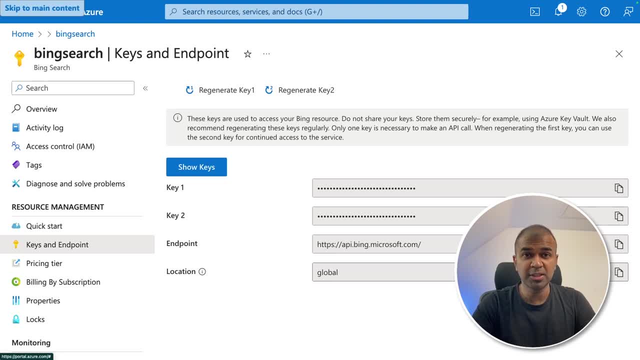 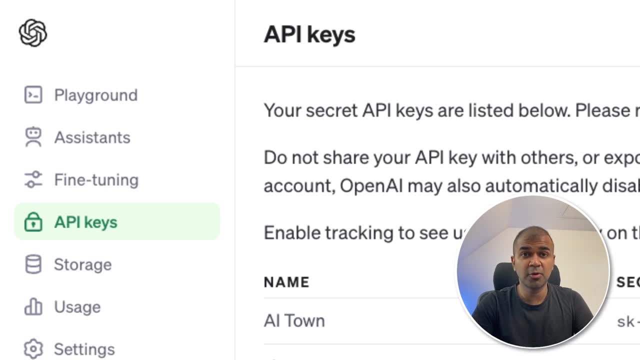 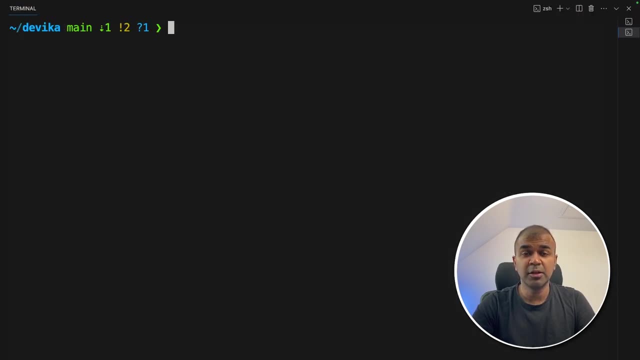 So this Bing API is used for browsing the internet or searching. Similarly, if you go to platformopenai, you should be able to create API keys for OpenAI. In consoleanthropic, you can get API keys for cloud Once. after you modify this, save the file. You don't need to. 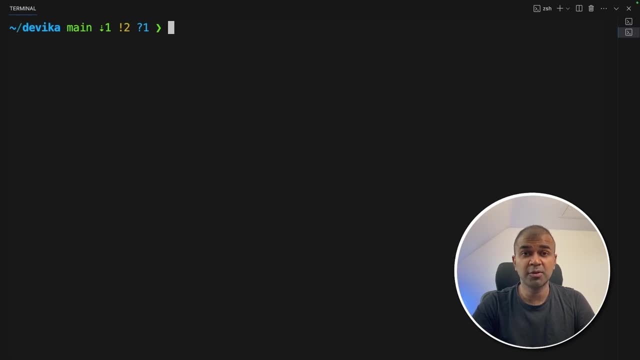 use cloud or OpenAI at the same time. You can use one of those, whatever you prefer Now in your terminal, pythondevikapy, and then click enter. This will automatically start the backend flask application. So keep the terminal running. Let's open a new terminal. Navigate to. 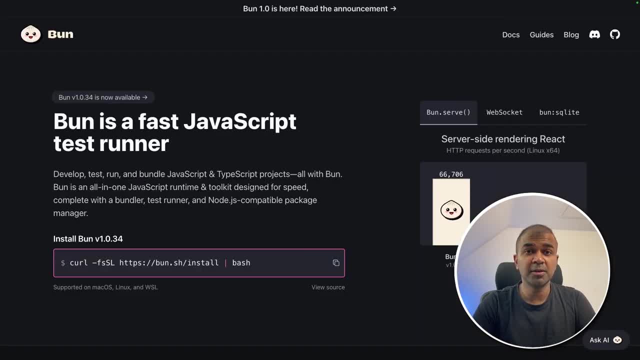 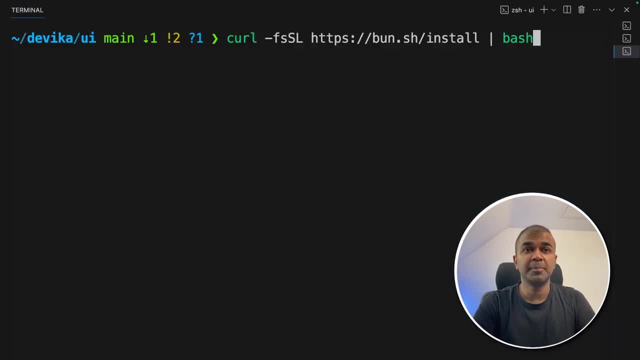 UI folder, cdui. Now we need to install bun to set up your frontend application. It is using JavaScript, So I'm going to copy this code to install bun and paste it here and then click enter. Now it's installing bun and it has been installed Now inside the UI folder, as you can see here. 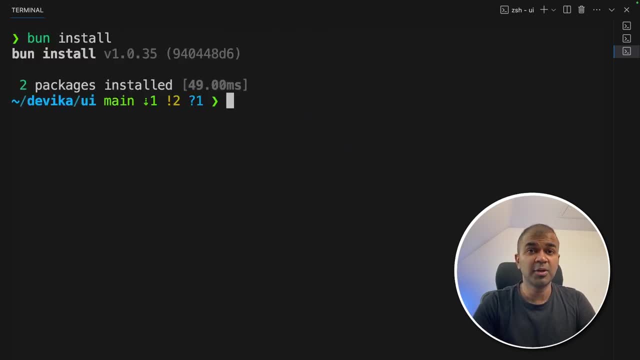 just type bun install and then click enter. I've already installed before, so it says I'll reinstall Now. bun run dev and then click enter. This will automatically start the frontend. Now you can open this URL and here's the interface. You can go up and create a new project. 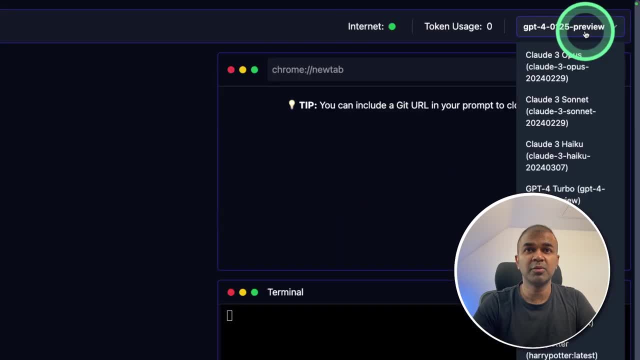 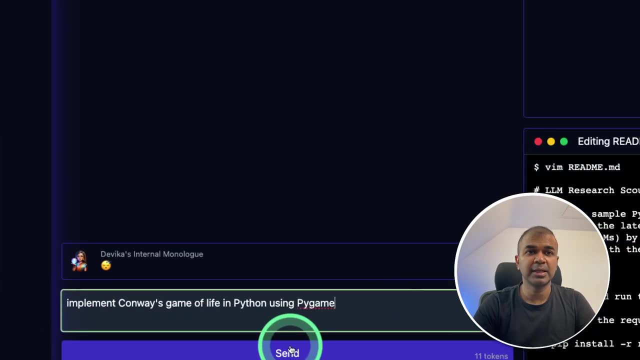 Let's say, test project. Now we need to choose the model we want to use. I'm going to use GPT-4.. So now going to ask: implement Conway's Game of Life in Python using Pygame and then click send. Now you can see on the left hand side you can talk to the AI engineer and here you can see it's. 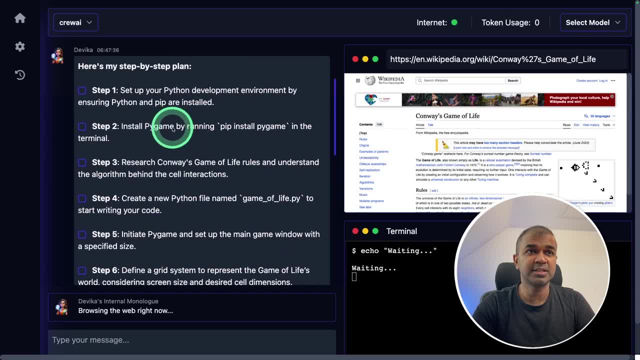 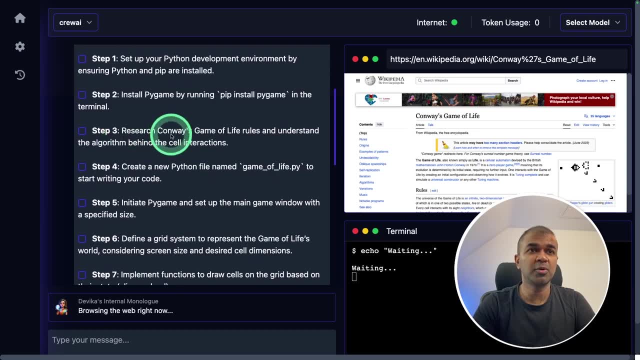 performing the request. It's listing all the steps on the left hand side. Here is my step by step plan: Set up a Python development environment. install Pygame research about Conway's Game of Life. So it's browsing in the right hand top corner. You can see that. Now it's going to the game development. 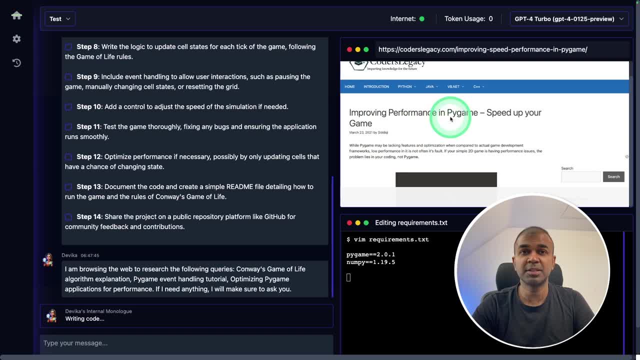 tutorial. Now it's researching the game development tutorial. Now it's researching the game development tutorial. Now it's researching about improving performance in Pygame. I can see at the bottom it's trying to run In the backend. you can see all the requests coming through Now in the readme.